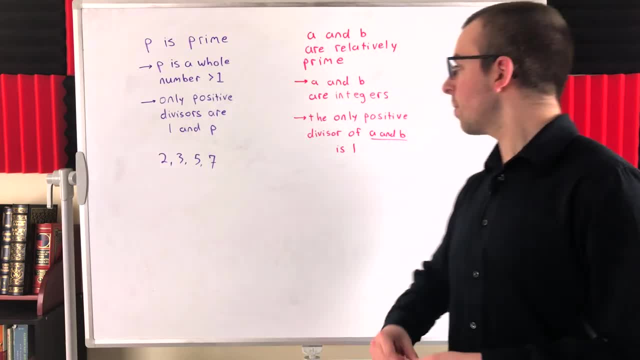 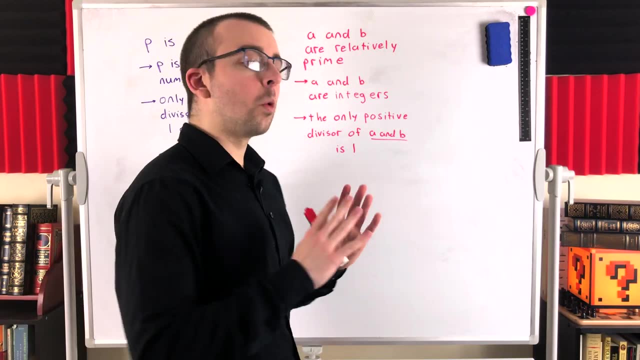 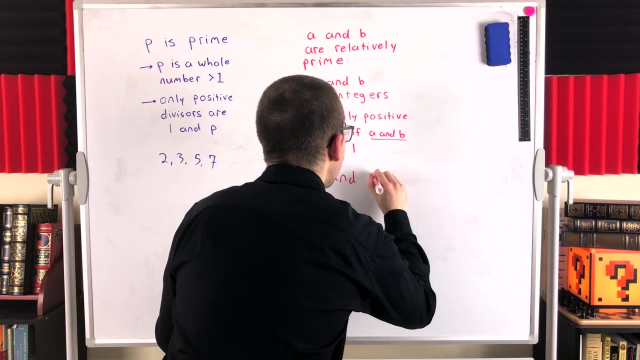 negative, two negative one, zero, one, two and so on. And the only positive divisors are the ones that are positive. divisor of a and b is one That means that one is their only common positive divisor. So, for example, the numbers four and nine are relatively prime. The positive divisors of four. 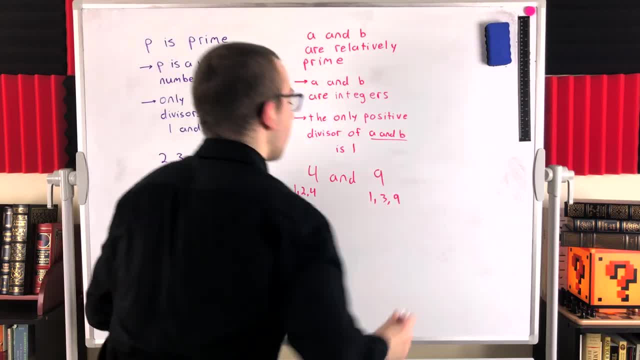 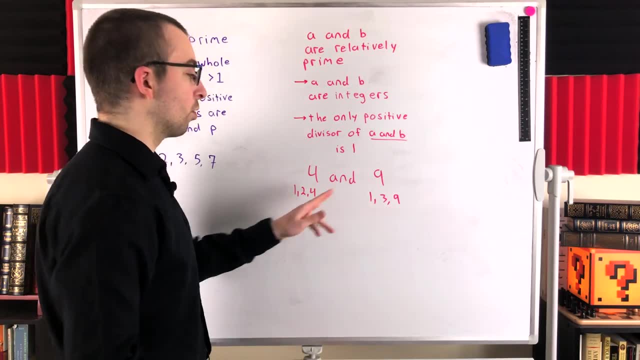 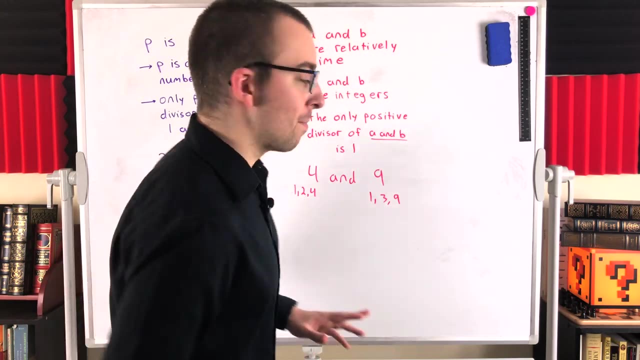 are one, two and four and the positive divisors of nine are one, three and nine. We see the only common positive divisor they have is one. So four and nine are relatively prime numbers. So what we see is that two numbers don't have to be prime to be relatively prime. We can also talk. 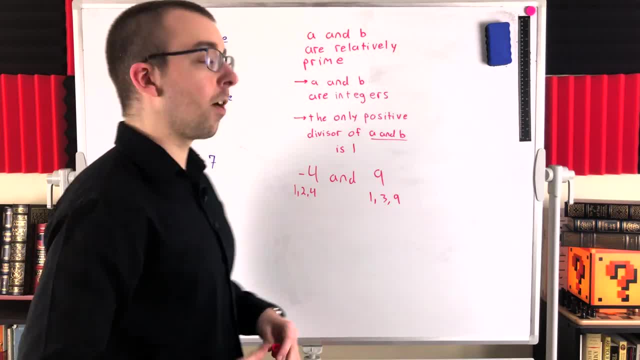 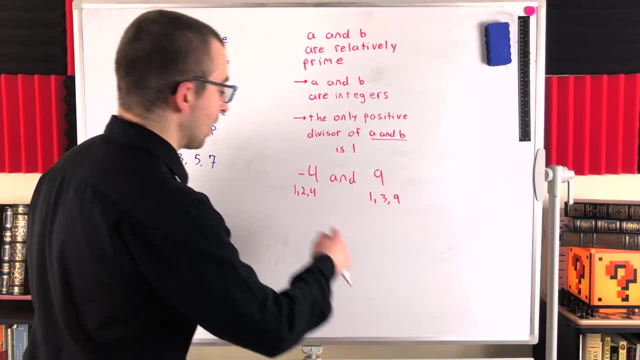 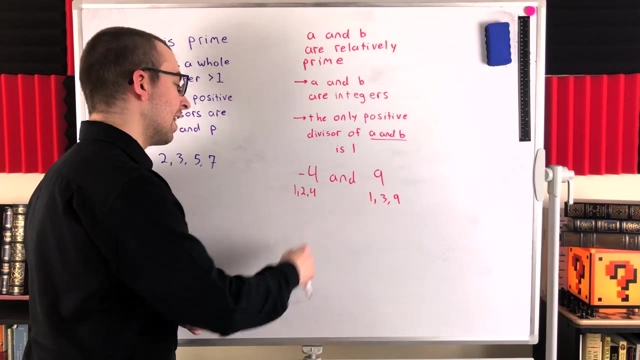 about this with negative numbers. Negative four and nine are also relatively prime, because negative four has the same positive divisors as positive four. We can multiply one by negative four to get negative four. We can multiply two by negative two to get negative four. And we can multiply four by 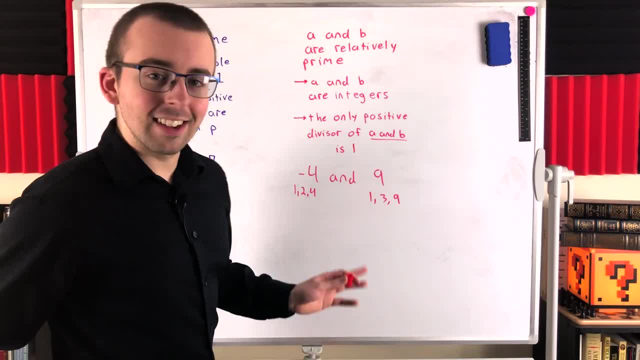 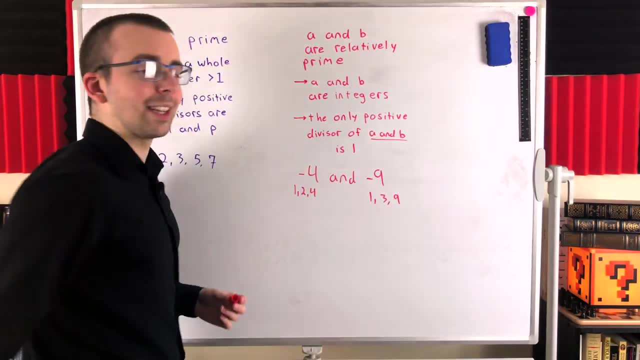 negative one to get negative four. So these are the exact same divisors as the positive divisors. So these are the exact same positive divisors for four or negative four. The negative doesn't change anything. Negative four and negative nine are relatively prime as well. Okay, so numbers don't. 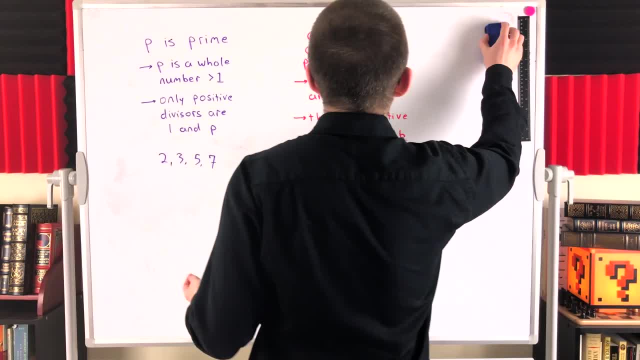 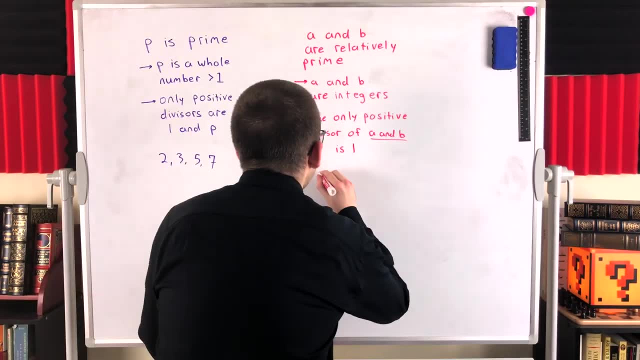 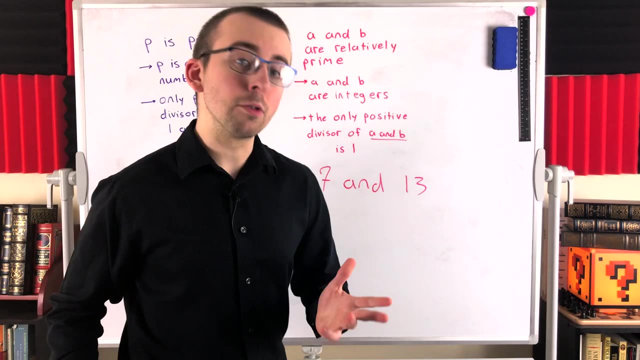 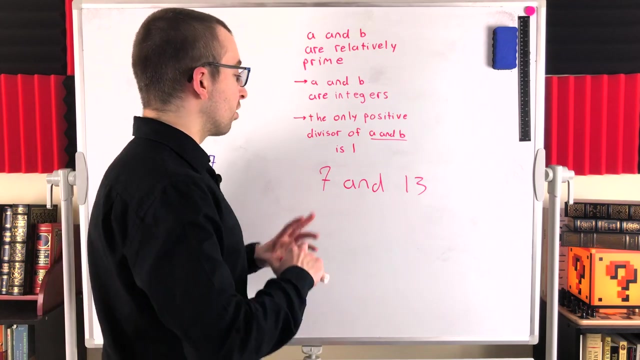 have to be prime to be relatively prime. But what if we are talking about prime numbers? How do prime numbers work with this relatively prime relationship? Well, certainly, if we have two distinct prime numbers, like seven and thirteen, they have to be relatively prime. If two distinct prime numbers had some common divisor other than one, then they certainly. 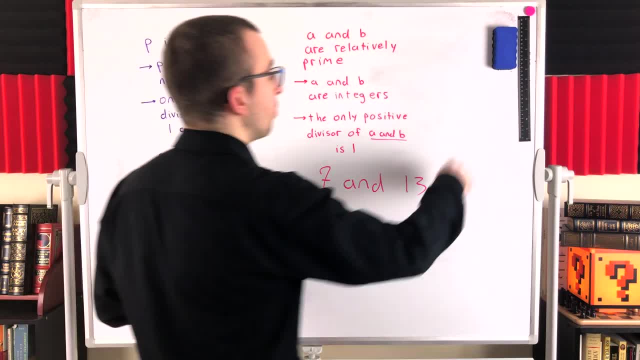 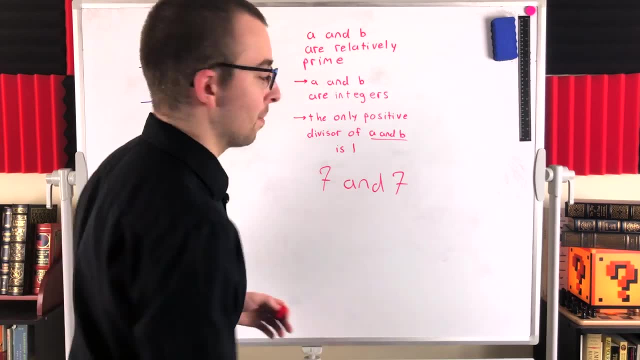 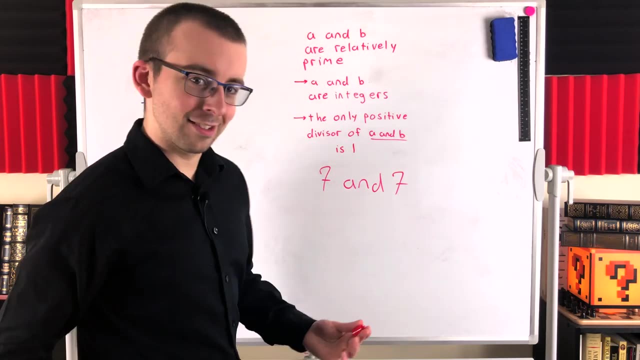 couldn't both be prime numbers. However, if we have two prime numbers that are the same, like seven and seven, then they are not relatively prime. Their greatest common divisor would be seven. Yeah, seven, I almost said one, It's seven. So if two numbers are relatively prime, that means their greatest. common divisor is 1.. 1 is their only positive common divisor, So let's say 7 and 14.. There's another example of two numbers that are not relatively prime. We saw that a prime number will always be relatively prime to any other distinct prime number. A prime number will never. 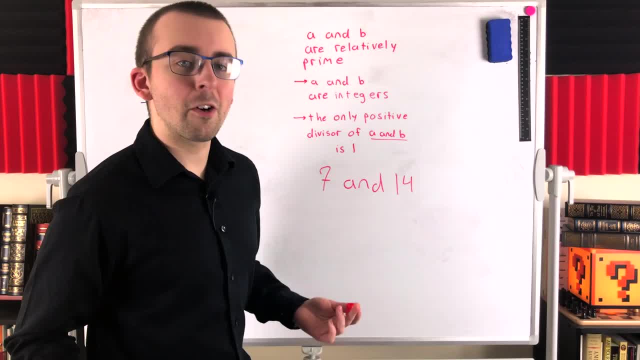 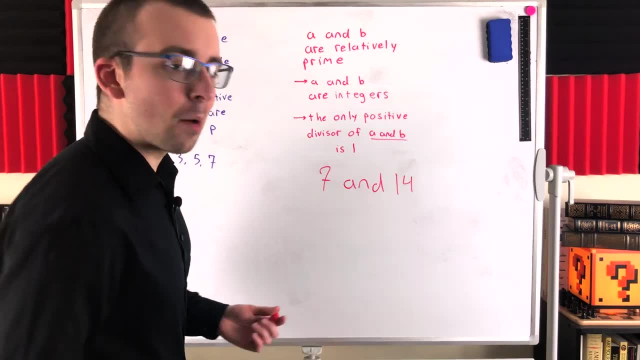 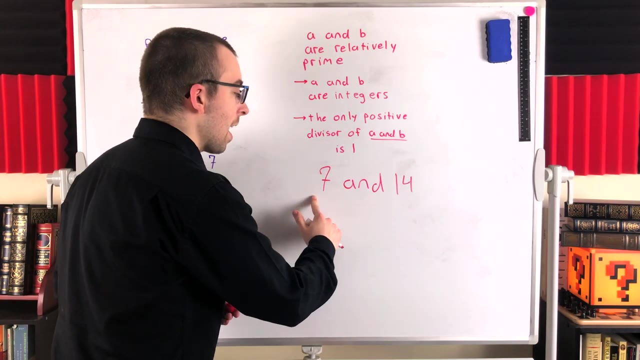 be relatively prime to itself, since they'll share a common divisor greater than 1 of whatever. they are right. 2 and 2 are not relatively prime. They have a common divisor of 2.. 5 and 5 are not relatively prime. They have a common divisor of 5.. But if we compare a prime to a composite, 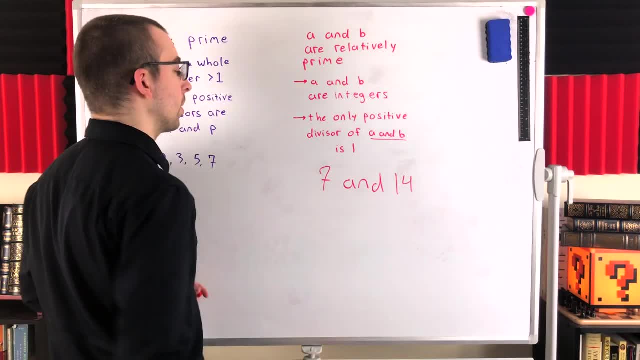 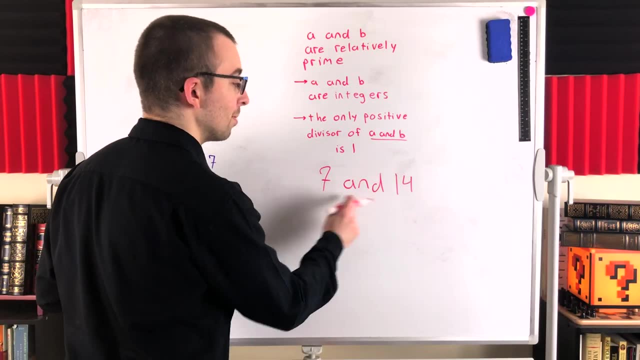 they may or may not be relatively prime. 7 and 14,, for example, are not relatively prime. Their greatest common divisor is 7.. 7 divides 7 and 7 divides 14.. But if we compare 7 to a different, 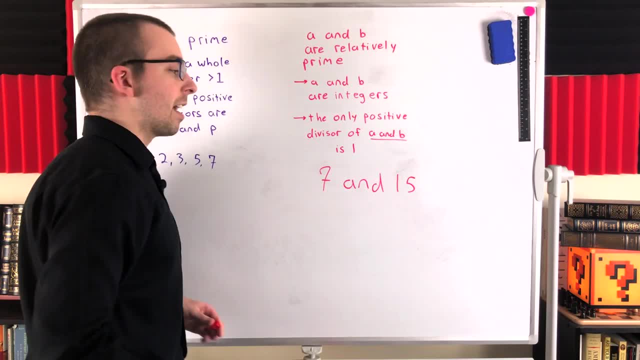 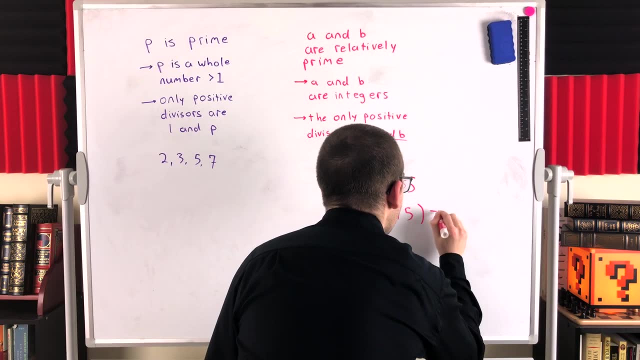 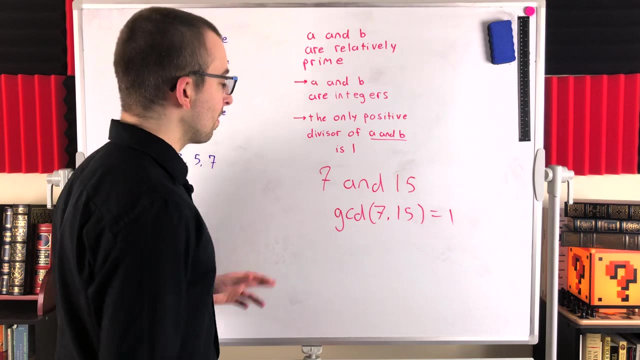 composite number, like 15,, for example. these numbers are relatively prime. The greatest common divisor of 7 and 15 is 1.. 15's positive divisors are 1,, 3,, 5, and 15.. And 7 does not share any of those except for 1.. 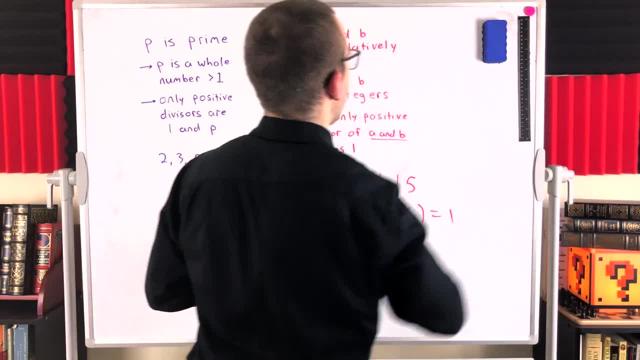 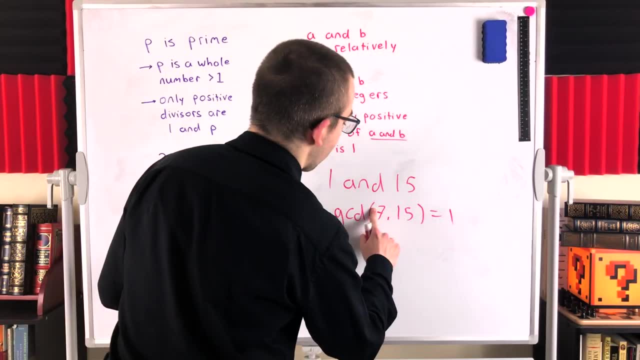 Now, what about, instead of looking at 7 and 15, just for another example, how about 1 and 15?? Are these relatively prime? They certainly are, because they are integers and their greatest common divisor is, of course, 1.. 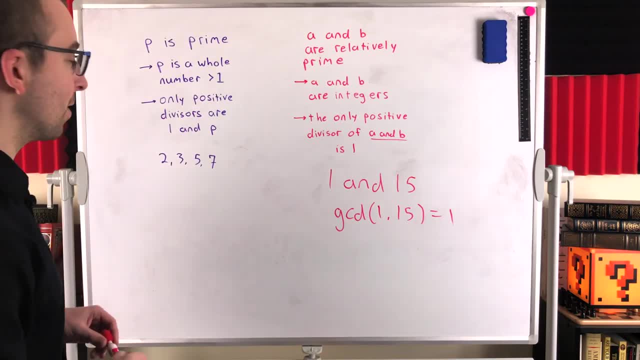 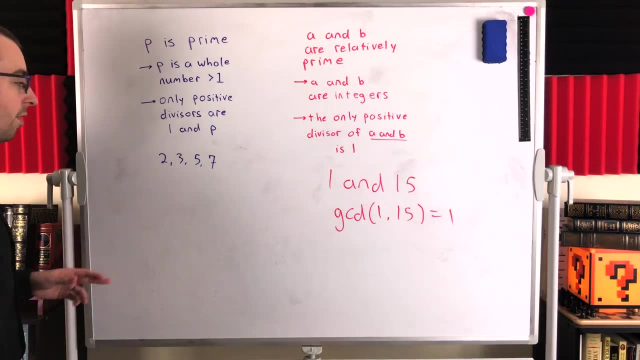 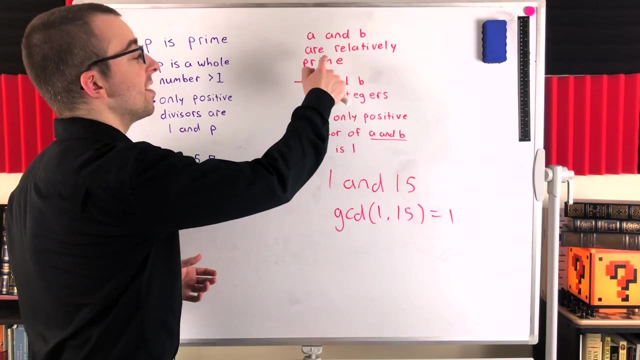 That's the greatest common divisor of 1 and 15.. So, as a quick recap, remember, a prime number is a whole number greater than 1, whose only positive divisors are 1, and itself like 5, whose only positive divisors are 1 and 5. We say that two numbers are relatively prime if they are both. 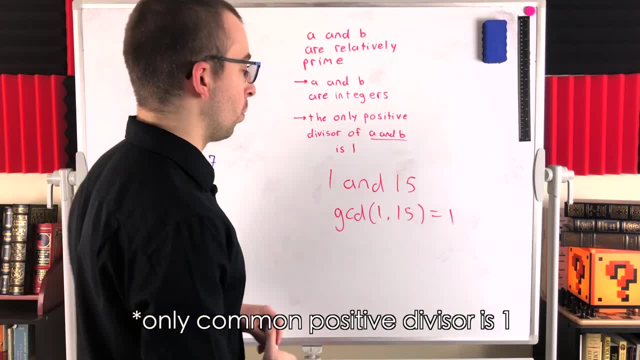 integers, and their only common divisor is 1 and 5.. So, as a quick recap, a prime number is a whole number greater than 1, whose only positive divisor is 1, like 1 and 15, or 7 and 15, like we looked at. 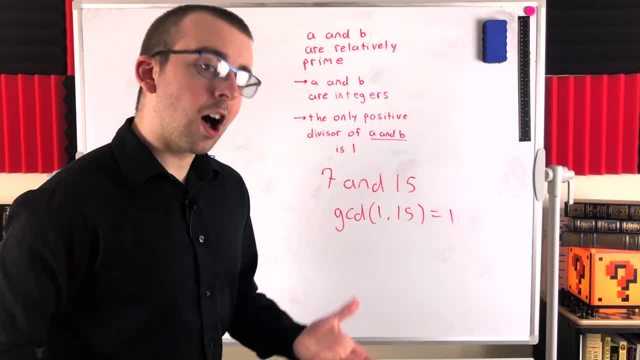 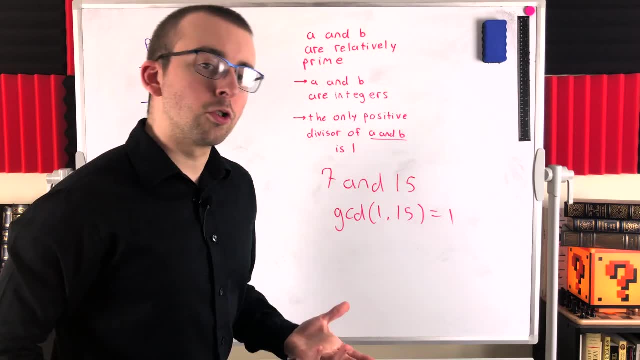 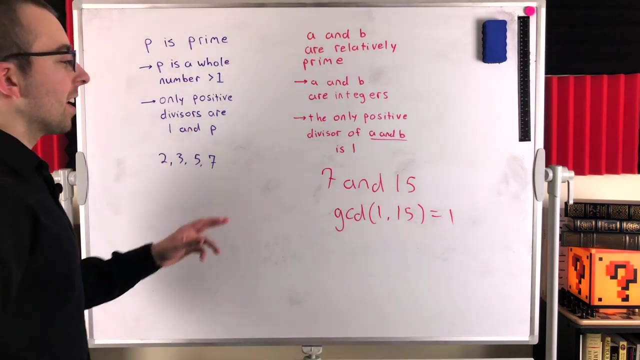 just a minute ago. These two numbers. their only common positive divisor is 1,, which also means- we could state this a different way- that two integers are relatively prime if their greatest common divisor is equal to 1.. Then to solidify and test your understanding of the concept of relatively: